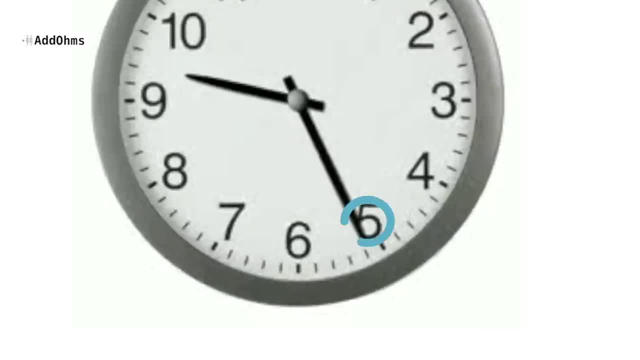 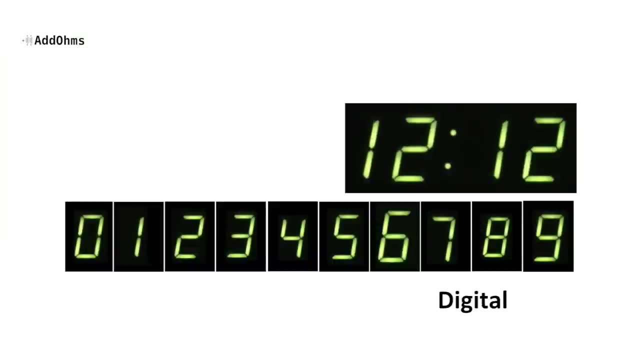 you can always tell how many minutes have elapsed just by looking at how far the minute hand is between the two numbers. When we look at a digital clock, all it can do is show us, for each digit of the time, the numbers zero through nine. 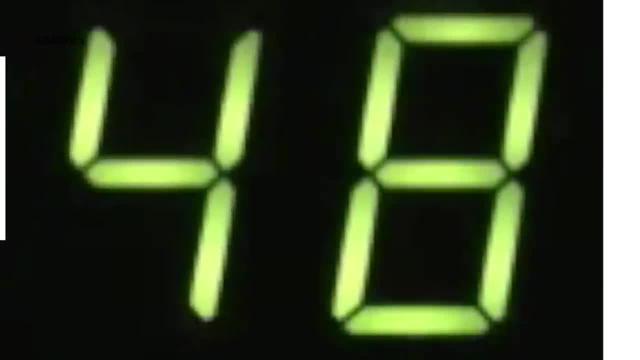 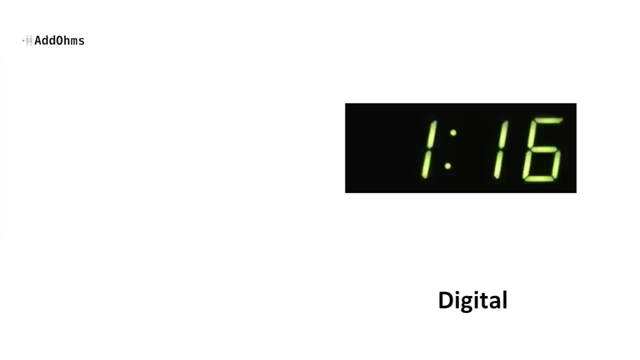 Even if we zoom in really really close, we can't see how close the clock is to flipping to the next digit. This means the increments of time are fixed to certain digits. Ok, ok, I know you're asking me: how does this all apply to electronics? 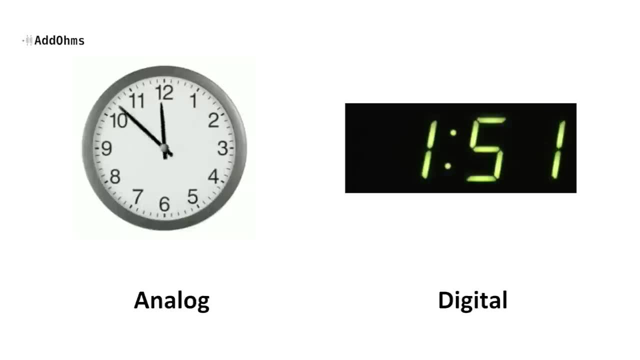 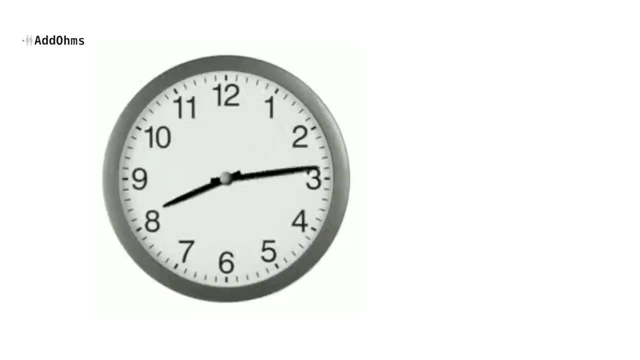 Let's use this to talk about analog electronics first. so As the clock's hands sweep across its face, the time displayed is continuously updated with nearly infinite precision. So even though we can see how close the clock is to the next digit, they can still. depending on where it's looking, which is a risky step. That doesn't mean they're gonna go back as many seconds, but they live their lives up to date after the clock. It even says something very panicky around maximum sensitivity with less than five seconds and even like you'd expect. 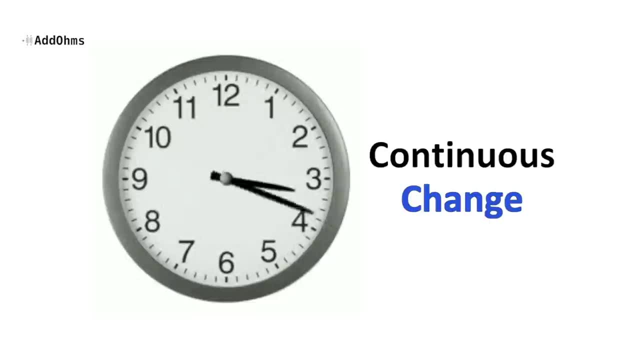 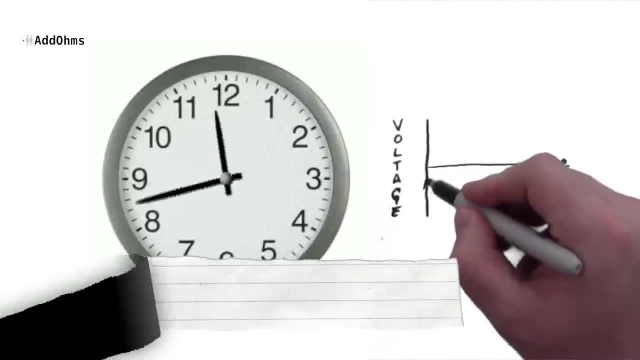 impetus, words over and over, Dang it, lose it. All these times give you such really high, continuous change. Analog signals are signals that are continuously variable, or in other words, continuously changing, just like the time on the clock, As we learned in the video on the difference. 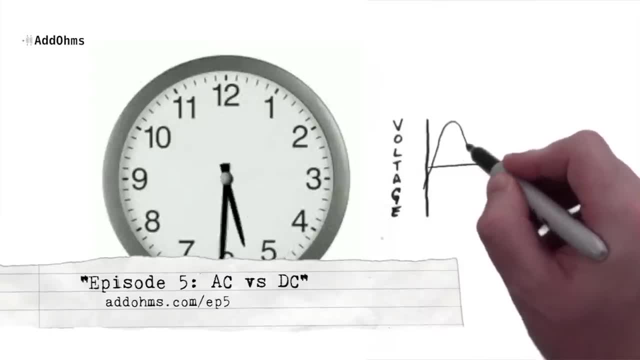 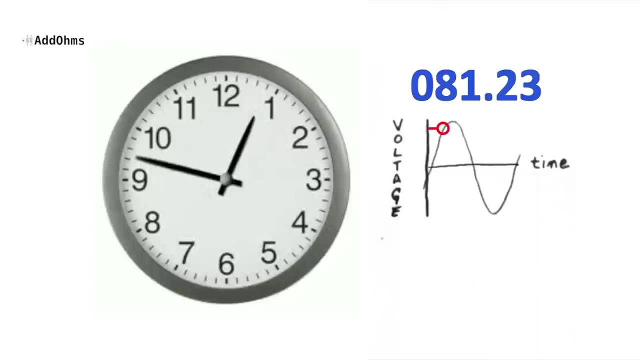 between AC and DC. the AC voltage in your house continuously changes at a rate of 50 to 60 hertz. Imagine that we had the ability to stop time and look at the voltage. Okay, I know bad pun, but what I wanted to show here is that, as we move across in time, that the voltage value is constantly. 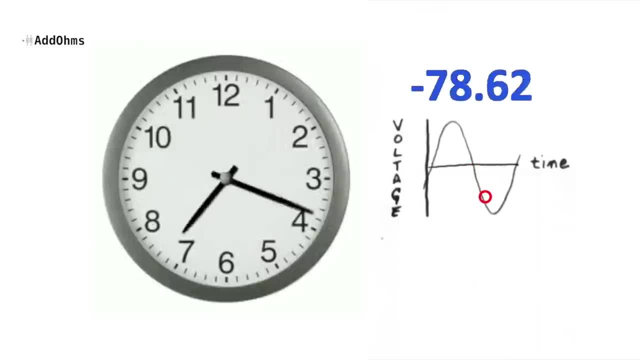 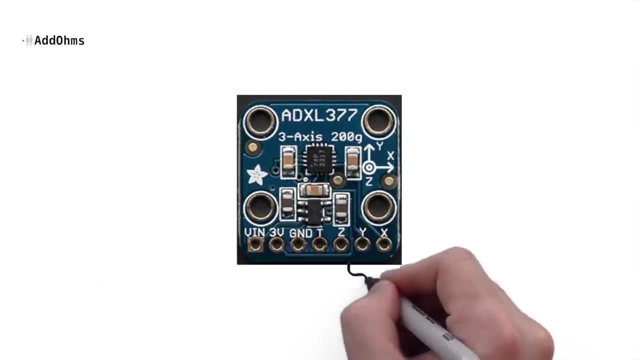 changing. This doesn't mean that analog is only found in the wall sockets or through AC. It's just a very good example. In fact, there are sensors like this accelerometer, which provides an analog output. This sensor varies its output voltage depending on how much acceleration is occurring. 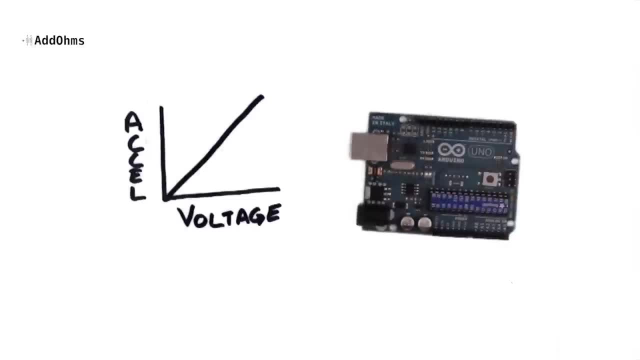 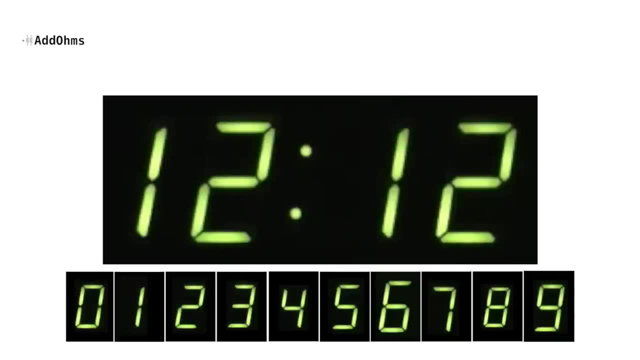 If you want to use that analog voltage with a digital system like an Arduino, then you're going to need to convert that signal to digital first. Going back to the digital clock, remember that time can only be represented by a fixed number of symbols, like zero, three. 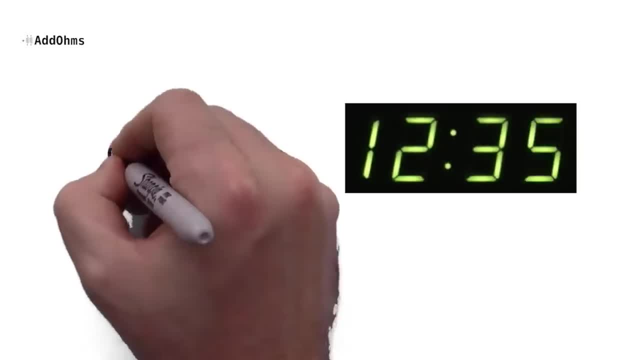 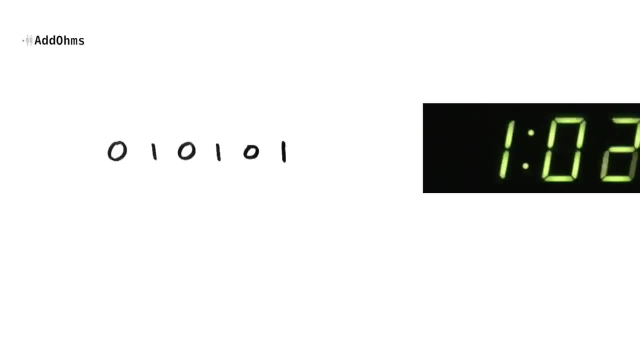 nine. The same thing is true in digital electronics. The digital signals can only be represented with fixed symbols like zero and one. But how do you get those zeros and ones? Well, it turns out that they're formed from voltage. Digital signals can have both a high level and a low level, and so what?